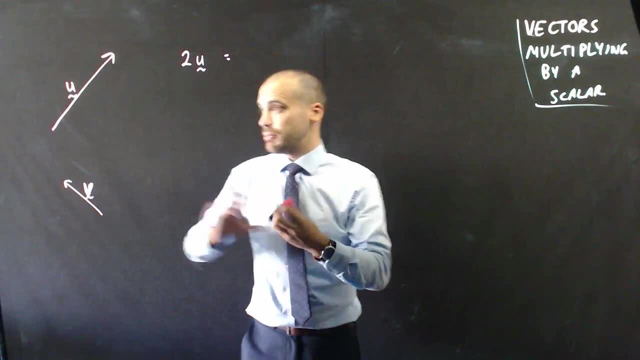 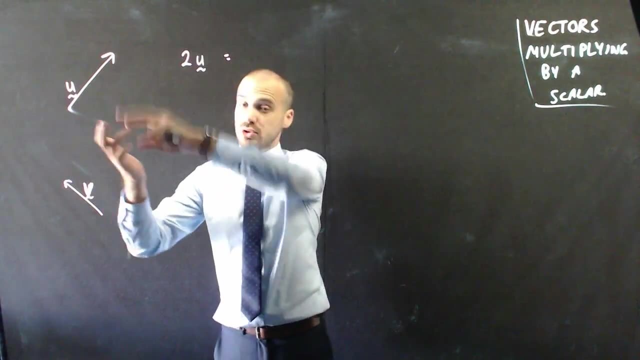 Okay, now vector 2u is just going to be. I might make u a bit shorter. You can probably guess why Vector 2u is still going to be in the same direction as vector u, but it's going to be twice as long. So it's about that long. 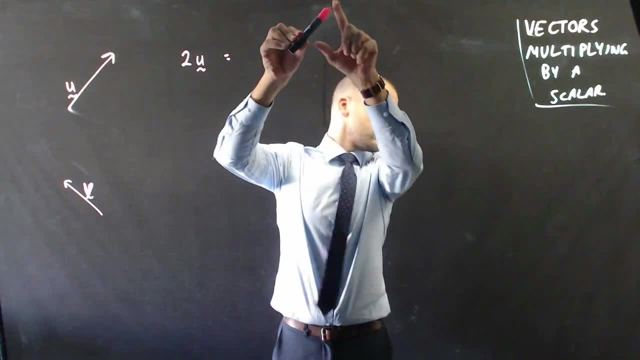 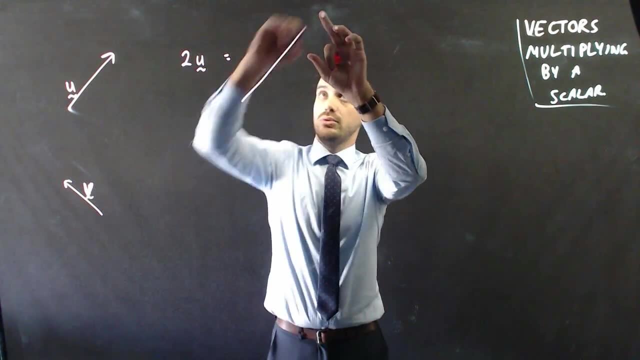 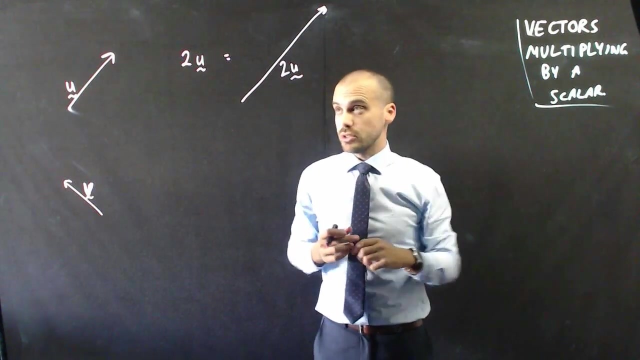 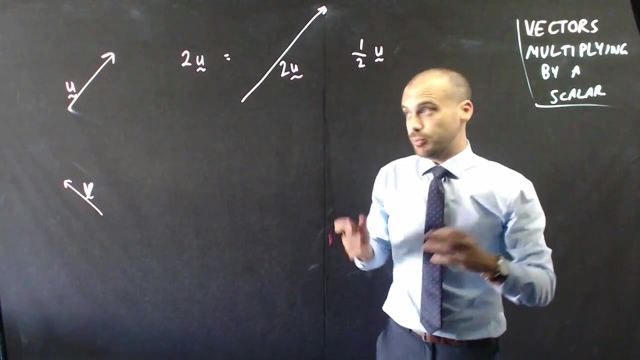 So, Hmm, Yep, Now I've lost my spot. Oop, oop, oop, oop. That is vector 2u. Same direction, twice as long. If I wanted to do vector half u, you could probably guess it's going to be half. 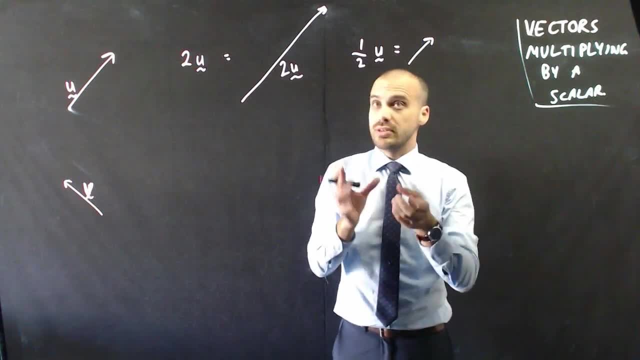 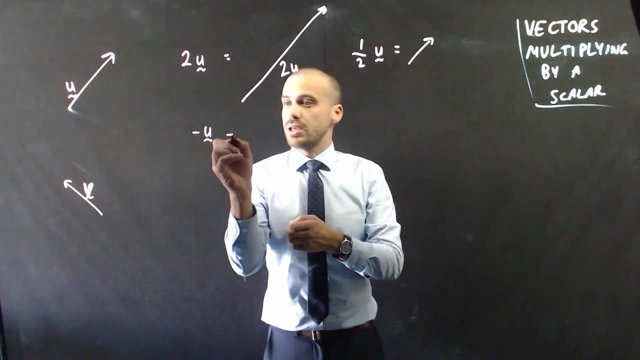 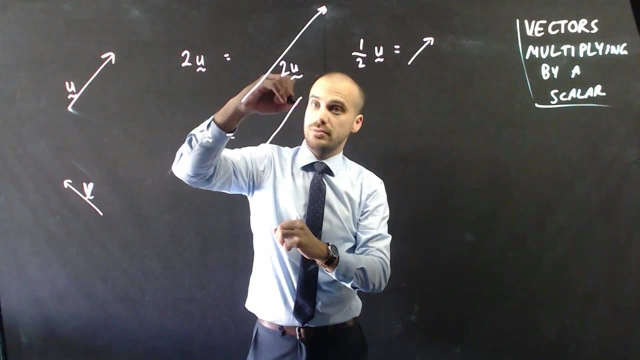 Now, if I wanted to do vector- We've already done this one actually- If I wanted to do vector, negative u or negative 1u, that's going to be equal to the same vector, but in the other direction. Same direction, but going in the opposite way. 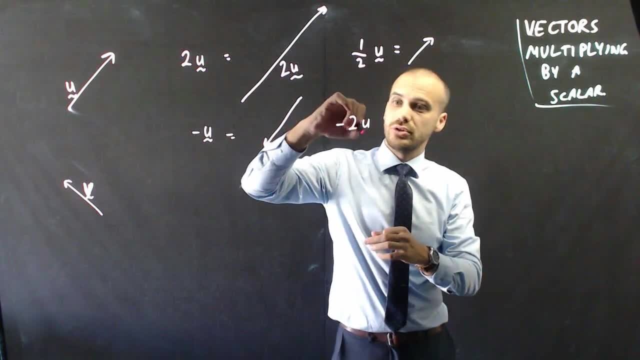 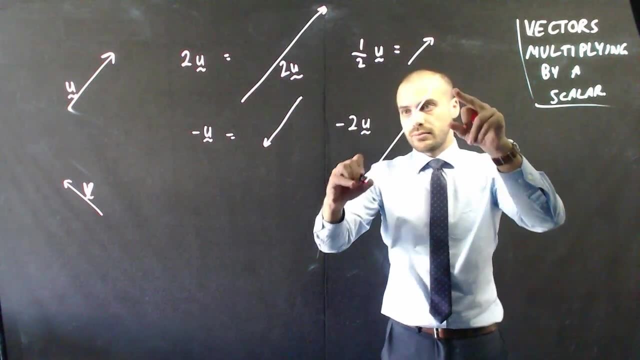 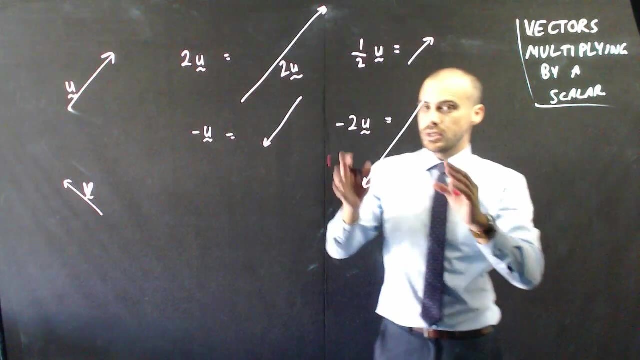 And now to combine those: if I want to do negative 2u, same direction, but backwards, and then twice the length, Okay, and that's vector negative 2u. So now that we've done that, I guess we could do one final step. 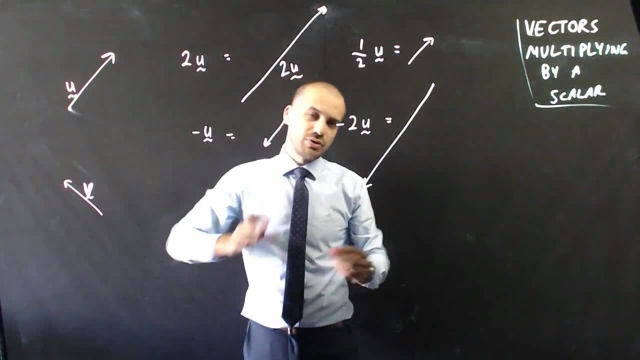 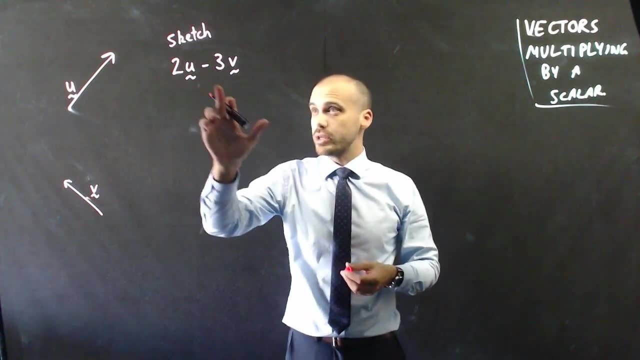 which is combine u and v, combine our knowledge of addition of vectors and also multiplication of vectors. So now we're going to sketch the vector 2u minus 3v. So what does 2u look like? Well, it's twice as long as that. We've already done this one. 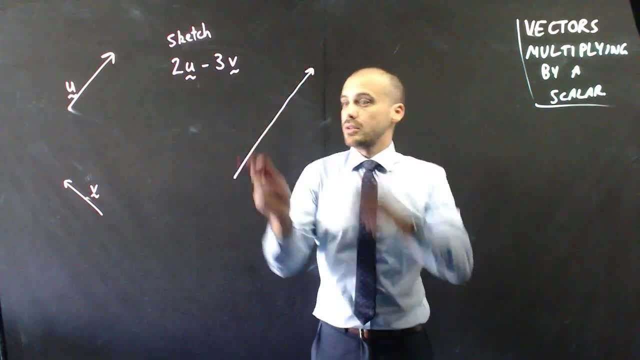 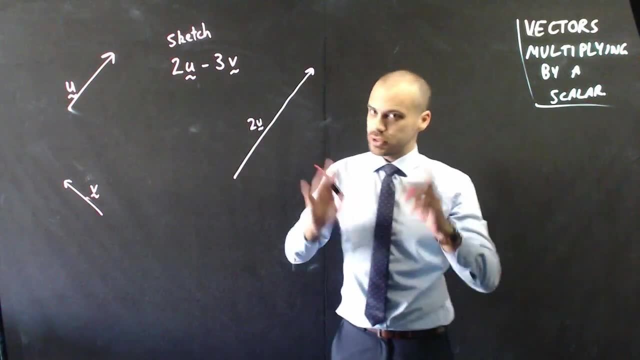 It goes from there Up to there. That's about twice as long as that. Good, That's 2u. Now negative 3v. I might just think about that for a minute. Negative 3v: This is v. 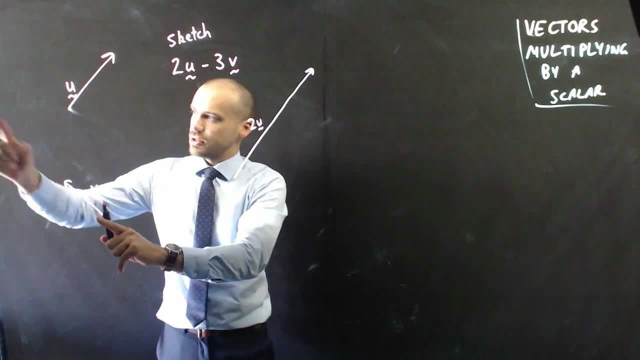 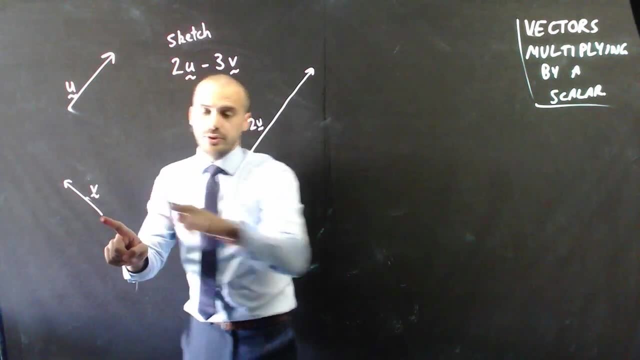 Multiplying it by 3 is going to make it 3 times as big. Making it negative 3v is going to turn it around. So it's going to look- I'll just draw it over here. It's going to look like that. 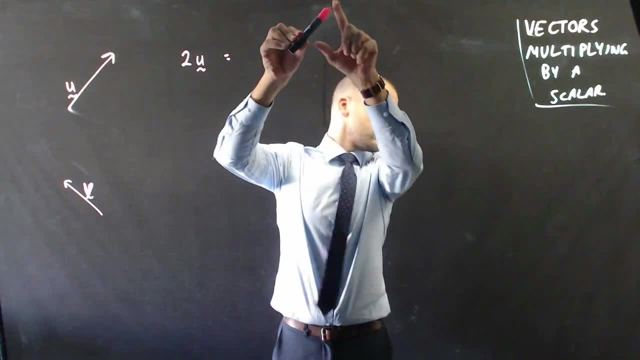 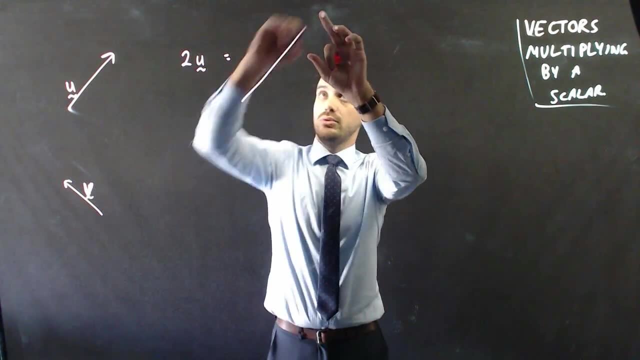 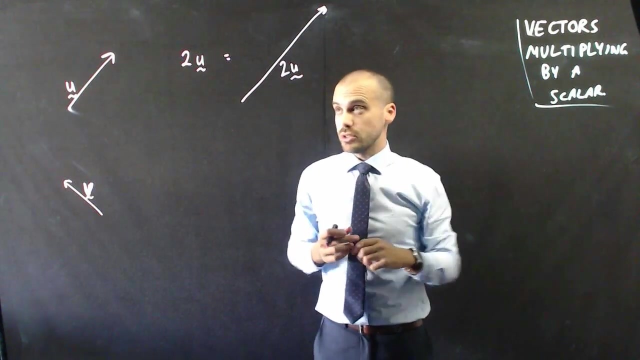 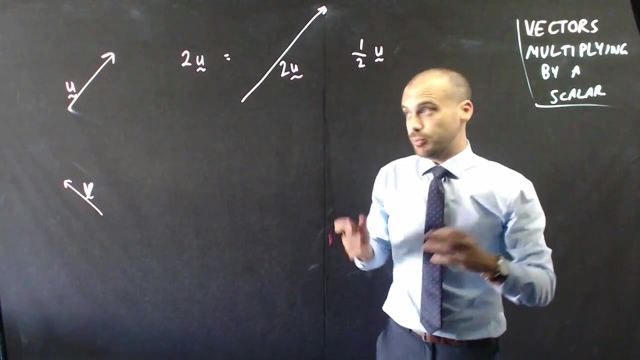 So, Hmm, Yep, Now I've lost my spot. Oop, oop, oop, oop. That is vector 2u. Same direction, twice as long. If I wanted to do vector half u, you could probably guess it's going to be half. 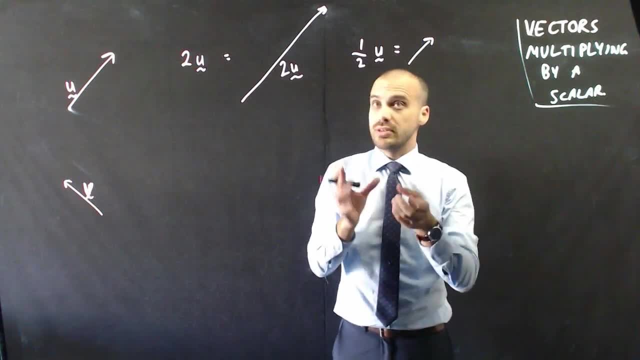 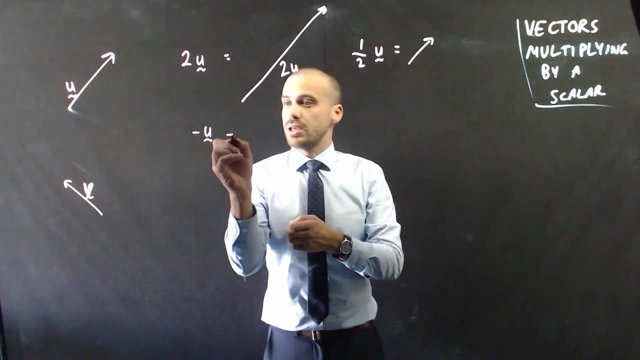 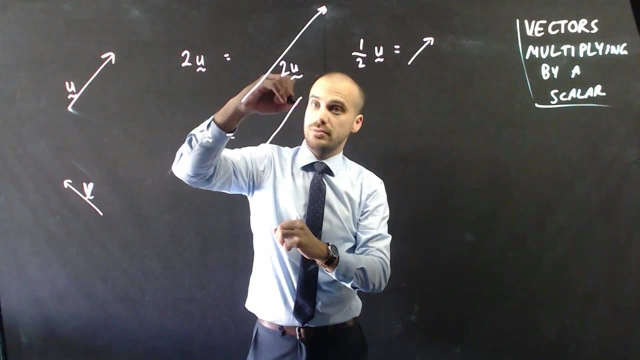 Now, if I wanted to do vector- We've already done this one actually- If I wanted to do vector, negative u or negative 1u, that's going to be equal to the same vector, but in the other direction. Same direction, but going in the opposite way. 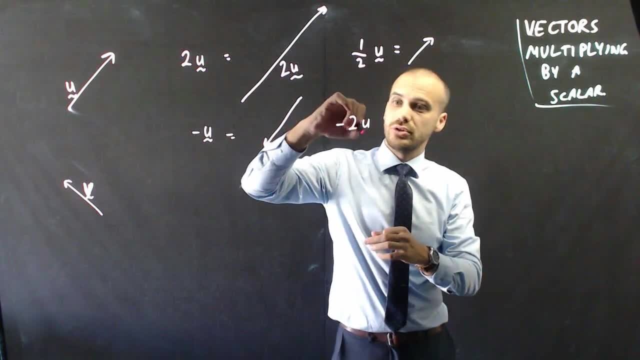 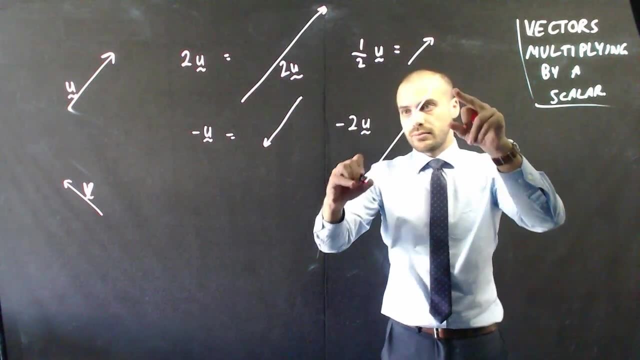 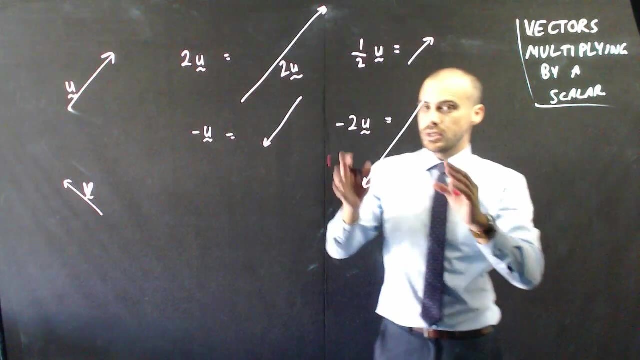 And now to combine those: if I want to do negative 2u, same direction, but backwards, and then twice the length, Okay, and that's vector negative 2u. So now that we've done that, I guess we could do one final step. 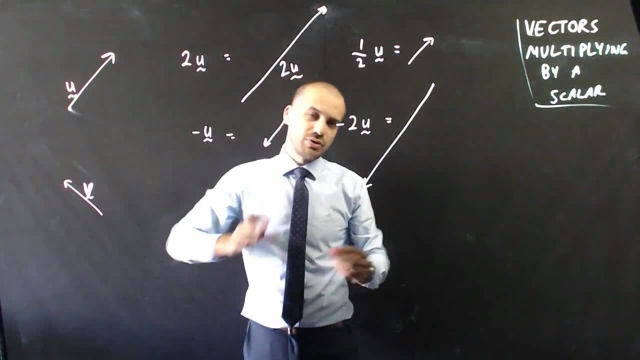 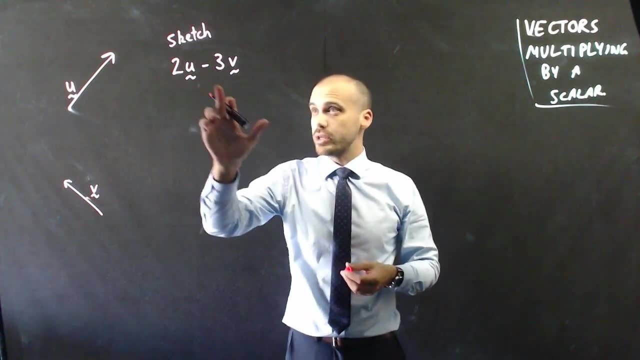 which is combine u and v, combine our knowledge of addition of vectors and also multiplication of vectors. So now we're going to sketch the vector 2u minus 3v. So what does 2u look like? Well, it's twice as long as that. We've already done this one. 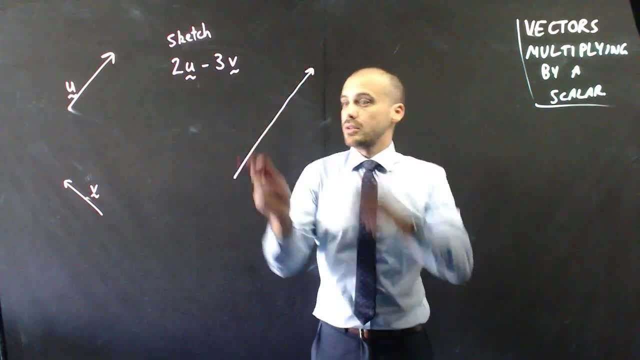 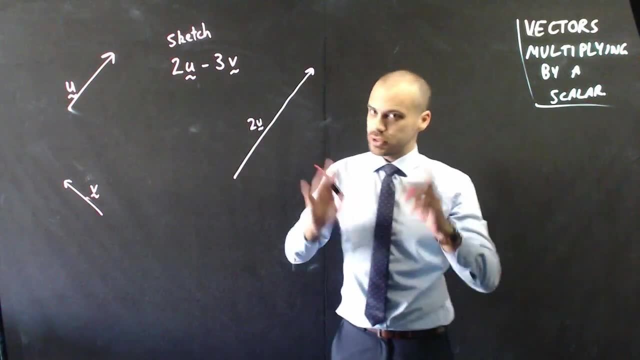 It goes from there Up to there. That's about twice as long as that. Good, That's 2u. Now negative 3v. I might just think about that for a minute. Negative 3v: This is v. 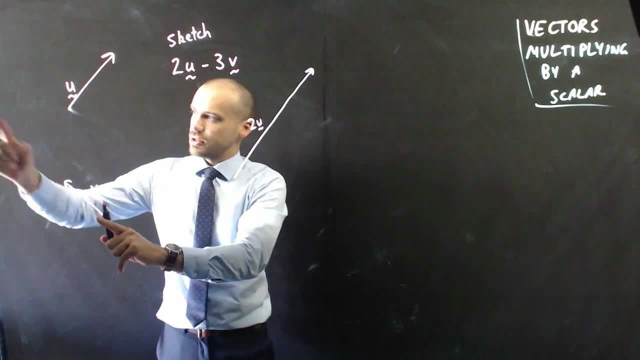 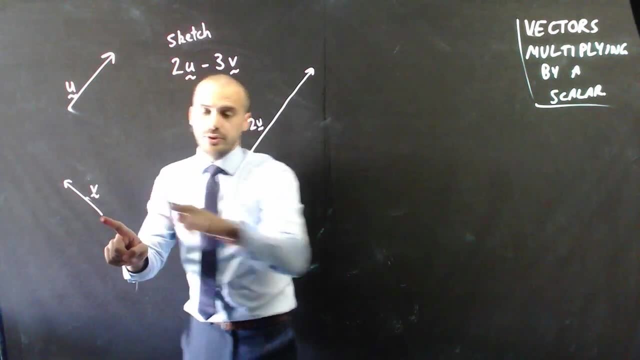 Multiplying it by 3 is going to make it 3 times as big. Making it negative 3v is going to turn it around. So it's going to look- I'll just draw it over here. It's going to look like that. 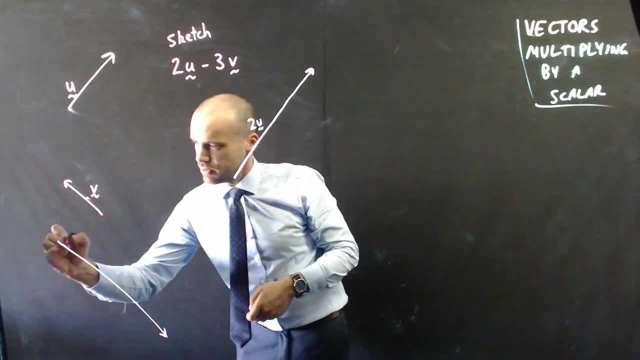 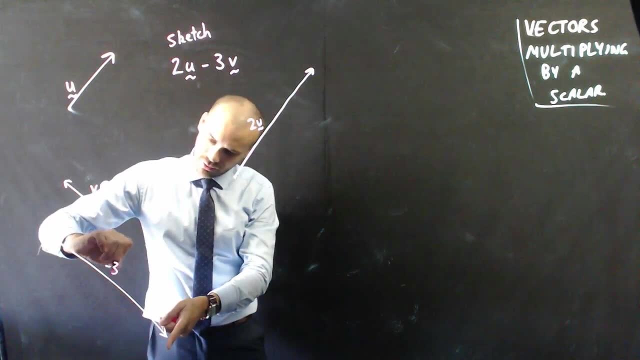 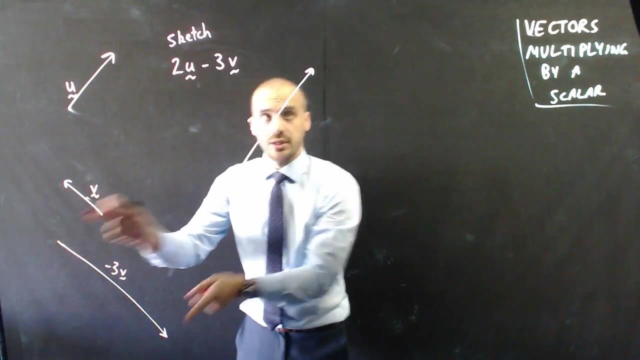 1, 2, 3.. That's about long enough. And going in the other direction. Now that's negative 3v And I'm going to take negative 3v and add it to 2u, which means I'm going to take the tail of it and stick it onto the head of it, like that.